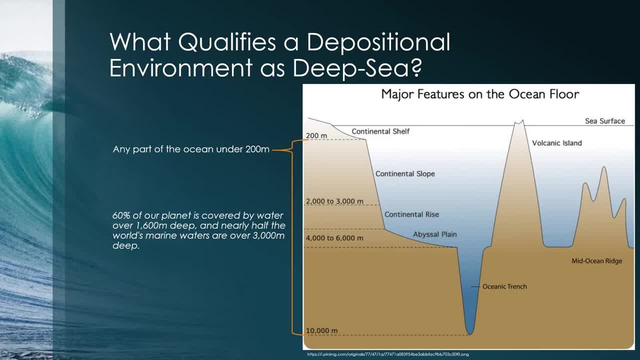 hydrothermal vents or biological sediment in the form of oozes. this muddy layer inevitably creates the flat appearance that we think of when we think of the ocean floor and is one of the most important parts of this depositional environment. There are two main types of sediment. 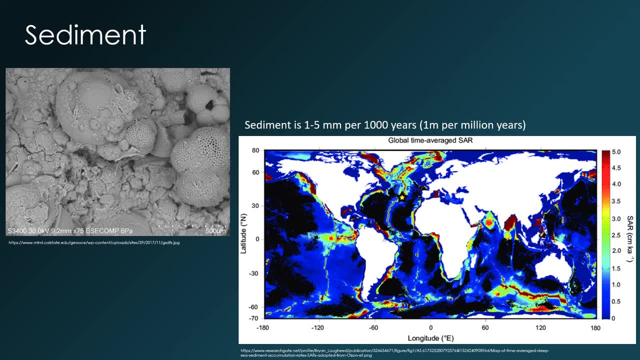 hemipelagic sediment and pelagic sediment. Hemipelagic sediment refers to the fine-grained sediment that comes from a continent. It consists of at least 25 percent non-biogenic material and has a few sub-classifications. If it is calcareous, there is more than 30 percent. 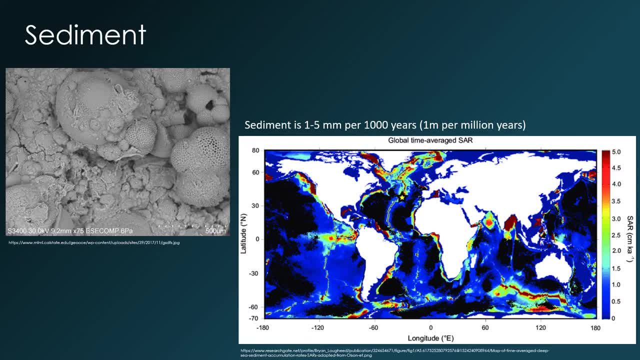 carbonate present. If it is terriginous, it is more than half weathered remains of land and less than 30 percent carbonate, And if it's volcanic, more than half of the sediment is volcanic in origin and again less than 30 percent is carbonate Pelagic sediments. on the other hand, 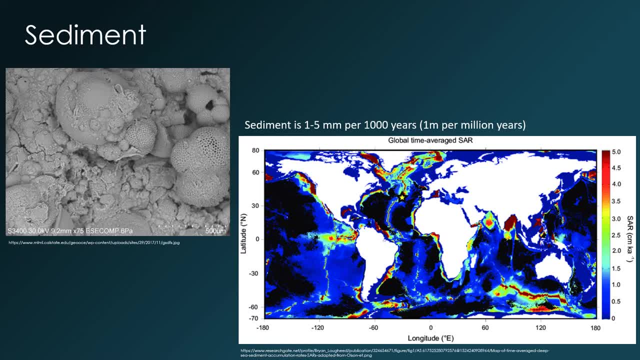 are made from the suspended material in the ocean and is comprised of terriginous dust, clay, silt, particles introduced by the wind, volcanic ash and some airborne particles from fire, which presents itself as carbon. There are also the remains of calcareous organisms such as 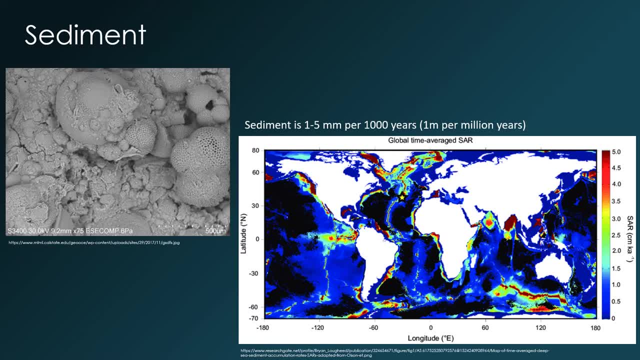 formentifiers, cockle bits, the skeletons of radularia and diatoms. These sediments collect once above deep, calm water and then settle, Since the terriginous material is often airborne when it is introduced to the water. it is also a source of carbonate. The sediment is also a source of. 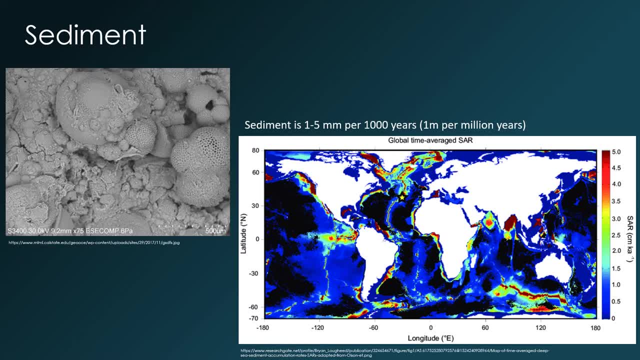 carbonate. The sediment is also a source of carbonate. The sediment is also a source of water. It typically comes from deserts or regions with loose sediment. This means that the particles are oxidized by the time they reach the ocean, creating a rusted looking color. Red clays are made. 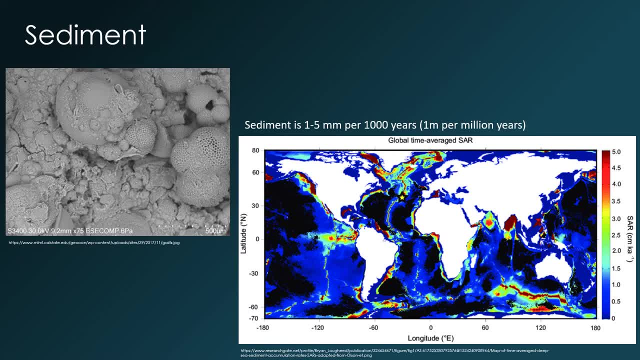 from 75 to 90 percent clay material and are rich in iron or manganese. This red clay will liphify and form red mudstone. Now this factor alone is important when it comes to looking at the defining aspects of deep sea oceanic activity. The fact that the clay is made from a deep sea oceanic 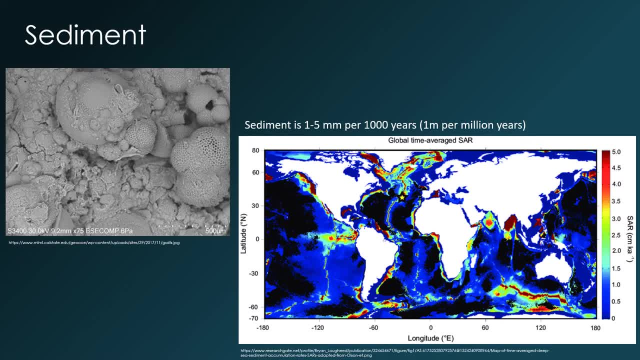 environment is important, Since red is not often a color associated with deep water environments. due to the basin-like shape of the ocean floor, the mud chert and mud limestone tend to create something resembling concentric rings, with the mud limestone closest to the continental margins. 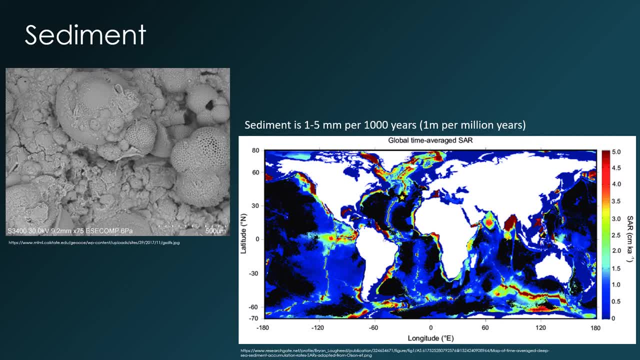 and the mud sediments farthest away. The rate at which the sediment accumulates is very slow, at only one to five millimeters every thousand years, Which means that it can take up to a million years just to create one meter of sediment. These types of sediment are most commonly biologic, as you can see from the top left. 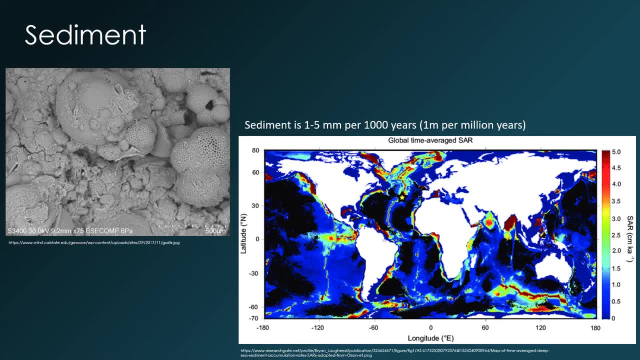 and the two groups of organisms which commonly make this up are formifaria and algae. Once the sediment settles and consolidates, it is often referred to as pelagic limestone. On the right you can see a map of how sediment settles over time and the most common areas which 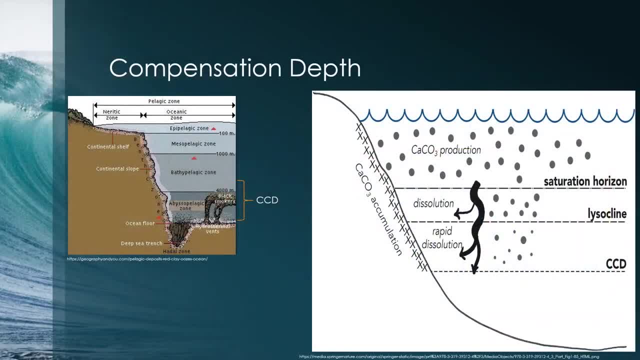 it settles. Before going to much into the sediments which fill this depositional area, I want to explain the depths where the sediments start to collect and go into solution. These depths are referred to as compensational depths and there are many different thresholds for different sediments. 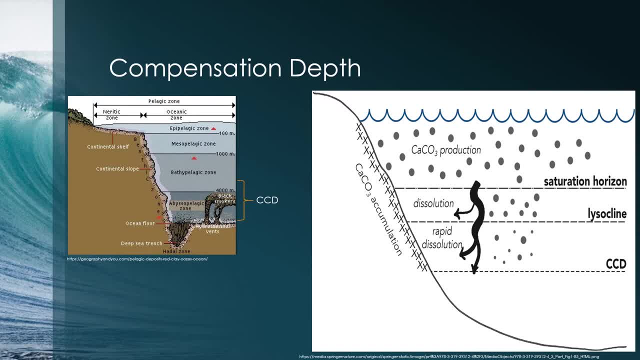 As you can see on the left, I have highlighted on this diagram about where the CCD, or compensational depths, would occur. Obviously, with temperature and pressure, these can change, but this is typically the case depending on the area that the sediment is deposited into. 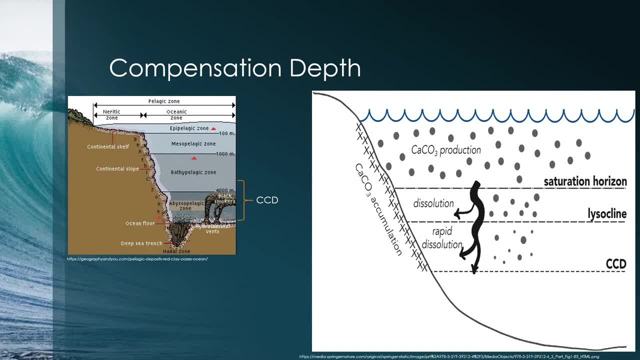 the range you will find them in. The one I will mostly be referring to from now on is the carbonate composition depth, or CCD. The threshold for this area is around 3,000 to 4,000 meters below sea level but, as I just said, can change based on factors like temperature, pressure and water. 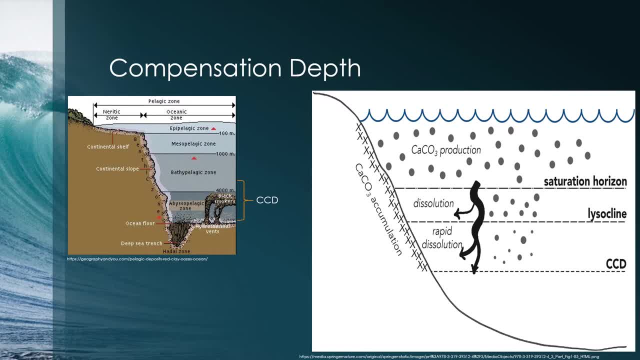 movement, as well as how much is already suspended in the solution. The more carbonate present, the deeper it will have to go in order to dissolve. Within this fluctuating range, the amount of carbonate added to the water is equal to the rate at which it dissolves. On the other hand, something 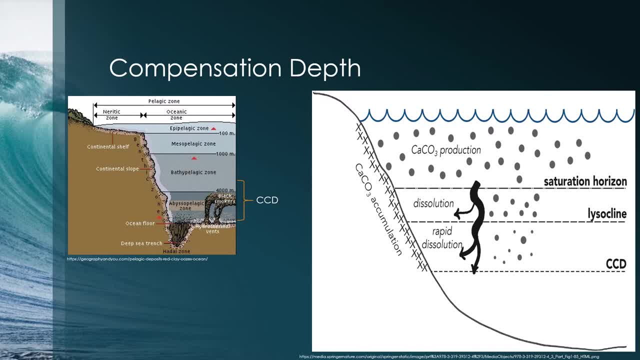 like opals, which are formed from skeletons of radiolarns and diatoms, is found much further down, at around 6,000 meters plus. due to the need for more pressure to dissolve, A sediment which is able to bypass this dissolution either does so by settling on a part of the floor leading down. 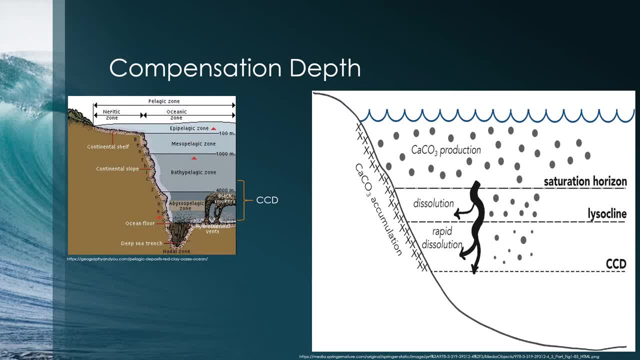 the floor or by a part of the floor leading down the floor. The amount of carbonate added to the this range, as you can see on the right, or because the water itself is too oversaturated or moving too much. this results in something called oozes. Interestingly, oozes form at a rate of 3 to 55. 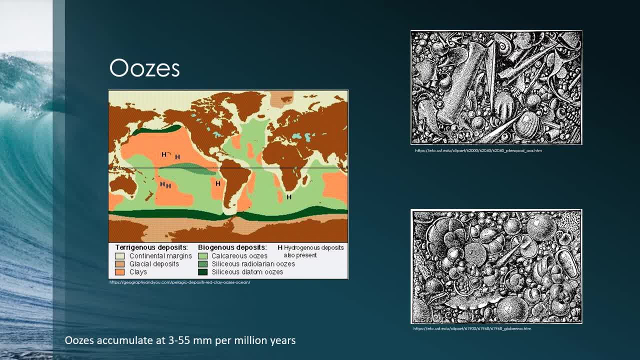 millimeters per million years, compared to the much slower 1 to 5 millimeters per million years of pelagic sediments. When it comes to oozes, there are two main kinds, this being calcareous oozes and siliconous oozes. Calcareous oozes tend to be found in warmer, shallower parts of the ocean. 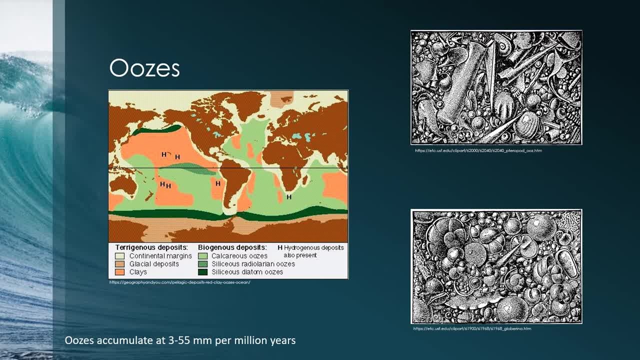 while siliconous oozes are found in more deep, colder portions. However, do not confuse these oozes with marine snow, as they do contain a lot of the same biogenous sediment from algae and formative area. Marine snow is simply the falling of these organisms, not the collection of them into. 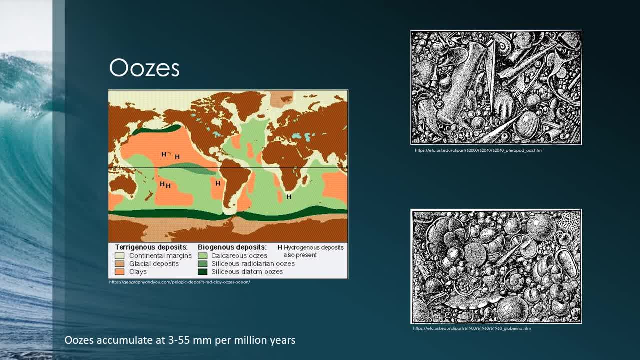 oozes. Calcareous ooze, as you can see from the light green, is what forms pelagic sediments. Siliconous ooze is a biologic limestone and is formed from the remains of coccolithophores or formative area primarily, which you might recognize, is what makes up chalk, Similarly to siliconous. 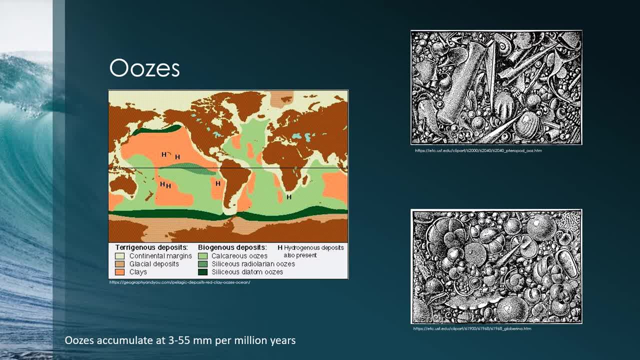 ooze. one of these two organisms, coccolithophores, requires sunlight, meaning it's found a lot closer to the surface, While formative areas do not and are found much lower in the ocean. as a result, As you would expect, there is more than one type of calcareous ooze. These include coccolithoos and. 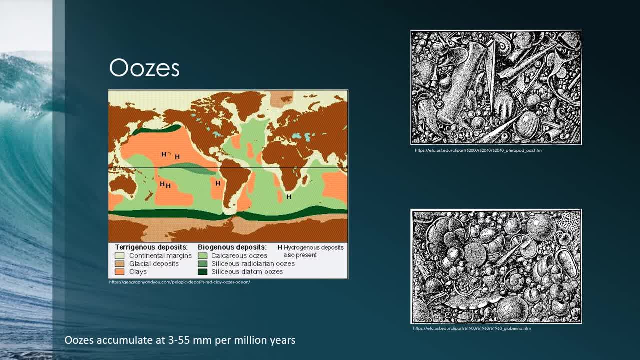 formative ooze, a subtype of that called globigaria ooze, and two other ones being petropod ooze and austropod ooze. Siliconous ooze, on the other hand, is made from the remains of diatoms and radiolarians. 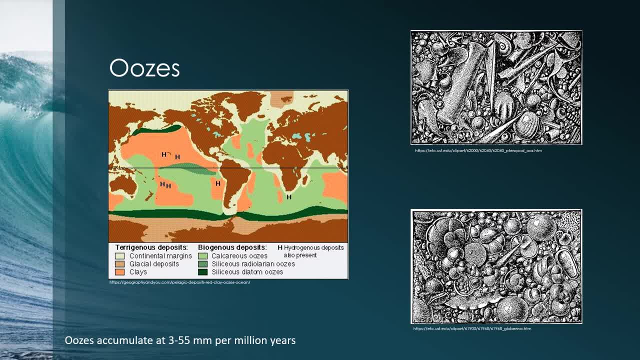 which are what forms. opal. Diatoms are an abundant microorganism towards the surface that collect in abundance on the ocean floor once they die. Radiolarians do not require sunlight, but do because of their ability to absorb the sun's light. Siliconous ooze is a biologic limestone. 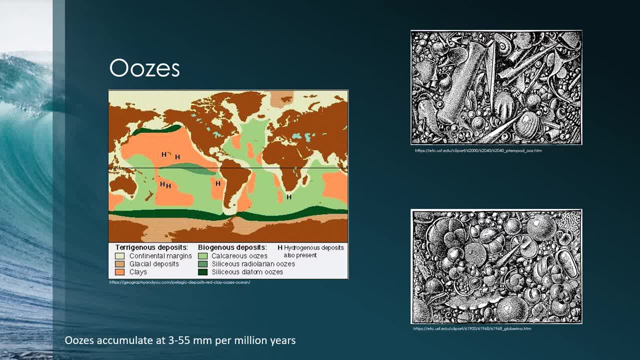 and, because of their symmetry, get the nickname snowflakes of the sea. I won't go into all the uses for diatoms in this presentation, but just keep in mind that they are a very useful organism outside of their environment and sedimentary uses. As with other sediments, this type of ooze has 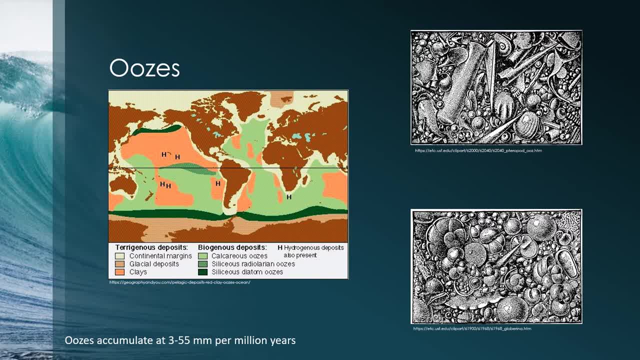 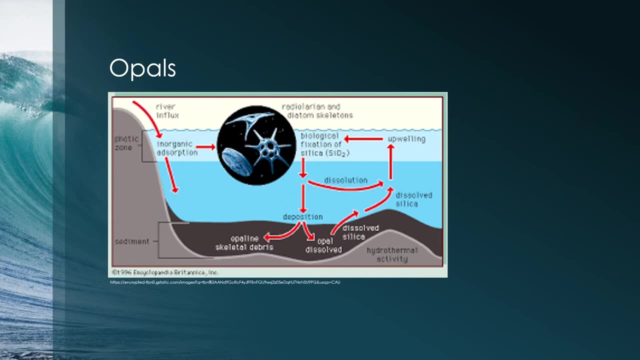 subdivisions. After the threshold of at least 30 percent silica secreting organisms, siliconous oozes can become diatomous oozes, radiolarian oozes and silico-flagellos. While siliconous ooze does come together to form opals, the opal created is often unstable. 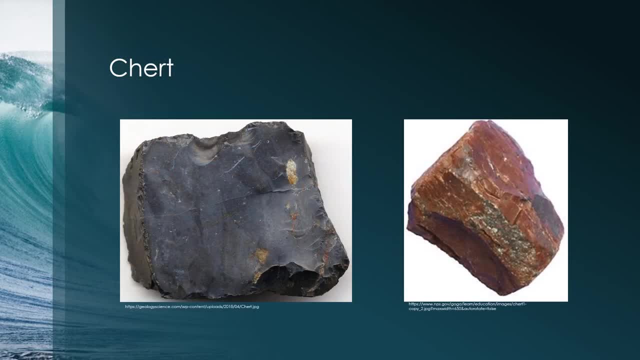 and alters to form what makes up chert. Chert is a fairly distinctive, often black or red rock. The black colour comes from the presence of carbon, while the red colour comes from clay. Both of these colors are good indicators of what formed the chert. However, there are other. 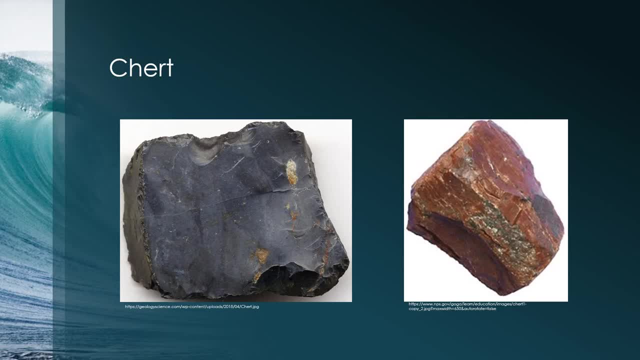 defining factors which help differentiate between types of chert. If radiolaria are present in the rock, it can be seen as fine white spots and causes the chert to be referred to as radiolarian chert. The beds this type of chert forms from are created by the lithification of silicon effuses. 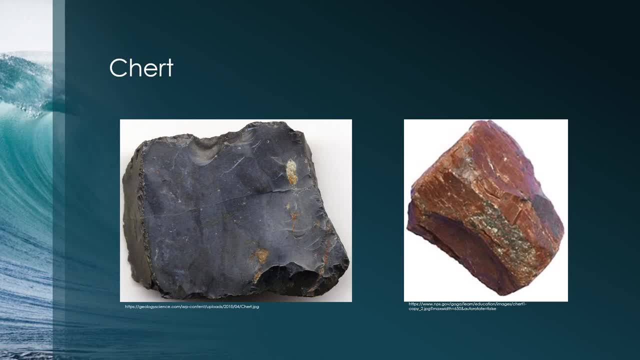 deposited in the water. Outside of this, there is also primary and secondary cherts. Primary chert is directly from the seafloor, with little to no other sources of sediment. Secondary cherts, on the other hand, are caused from when chert is formed by a host sediment, usually a limestone. 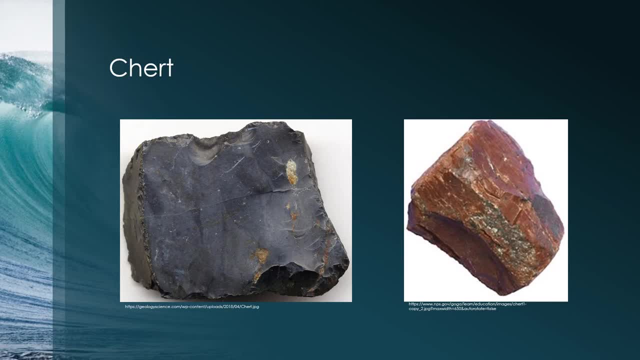 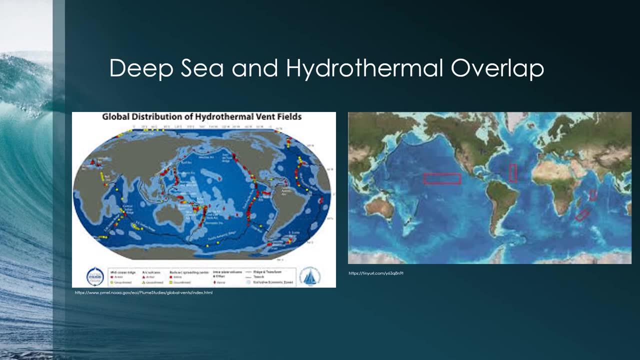 and tend to have an irregular shape. Before I explain the final kind of sediment, that being hydrothermal deposits, I just want to give a brief picture of how closely related the deep sea and hydrothermal areas are on this planet. On the left, you can see a map of all the hydrothermal. 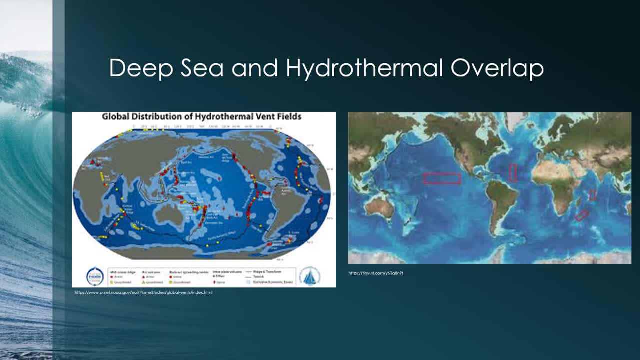 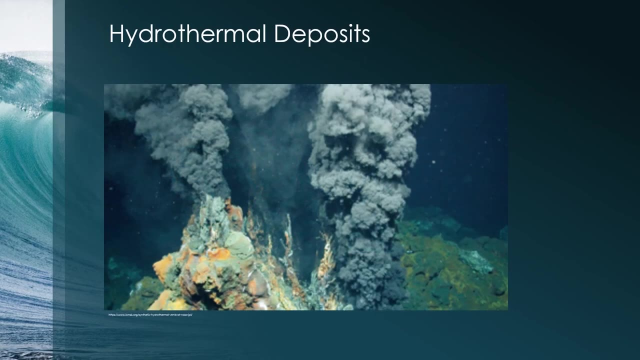 vents and on the right you can see from the darker blue where the deep sea tends to be located on our planet. As you can see, these do overlap quite a bit and definitely play a part in creating this depositional environment. I can 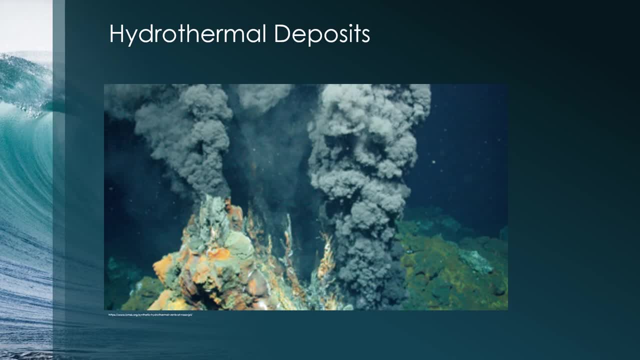 see that there is another source of sediment and deep sea invariants, as I had just mentioned: hydrothermal deposits. As you might imagine, hydrothermal vents are the sources of these deposits. Hydrothermal deposits are found around hydrothermal vents as a result of minerals being 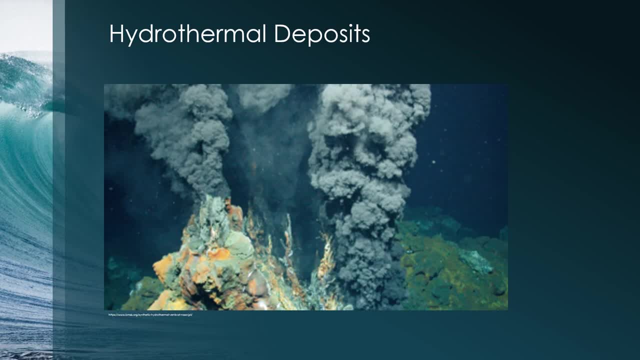 precipitated into the water by the heat produced. The water then cools enough, once reaching the seafloor, that it precipitates the minerals back out of solution, creating localized deposits around the vents. Black smokers are iron and sulfide rich vents, while white smokers are full of silicates composed of calcium and barium. 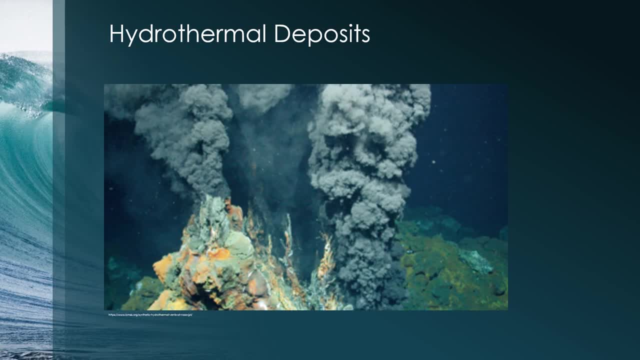 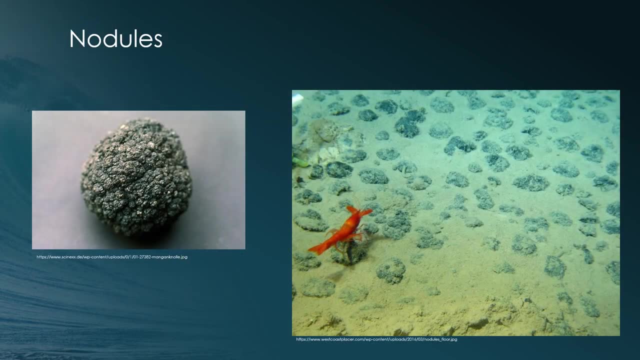 This collection of sediments often forms something called a nodule, or what is essentially a collection of metals on the ocean floor. So from hydrothermal deposits we can gather that nodules can be anything from iron to manganese, to barium or to calcium. However, there is another deposit that can also result. 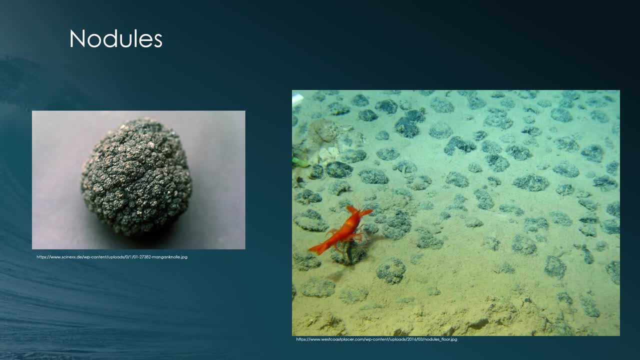 in nodules called hemogenic deposits. These occur in modern rocks as hard black rounded nodules, and these deposits include silicates, sulfates, sulfides and metal oxides, primarily iron and manganese. These metals in the deposit typically form from hydrothermal deposits. 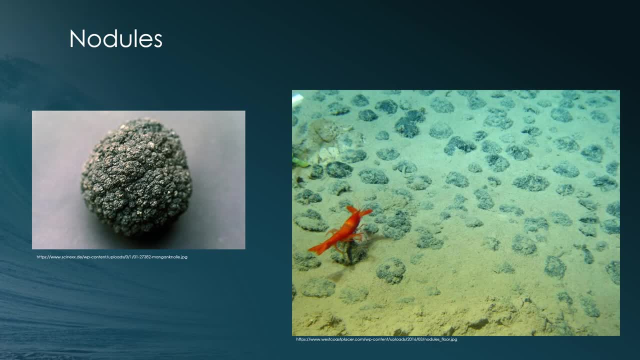 but can also be the result of continental weathering, including volcanic material. As I stated before, they can turn into nodules, given enough time, through chemical and biochemical reactions involving bacteria. However, at least for this type of sediment, it's an extremely slow process, at only one millimeter per million years. 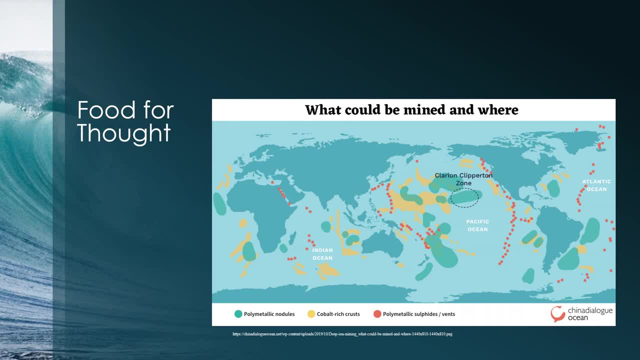 Knowing that nodules exist on the ocean floor and that they are comprised of metals, it is not hard to imagine the desire to harvest these resources. This is something already being explored around the world and, as you can see on this slide, China has mapped out possible locations to harvest certain minerals from. 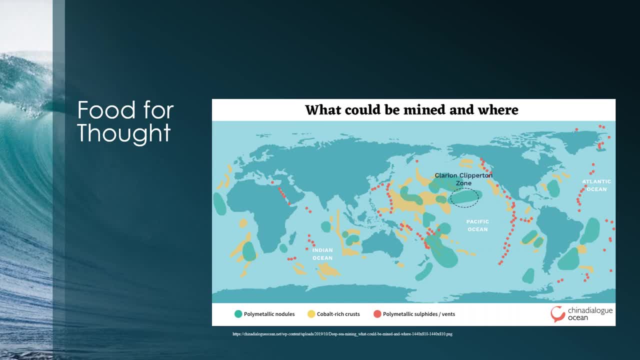 While this will not happen anytime soon, since there is a lot to learn and understand about these environments surrounding the deposits, it is important to consider that in the future, these areas may be harvested for their resources and because of that, it is definitely 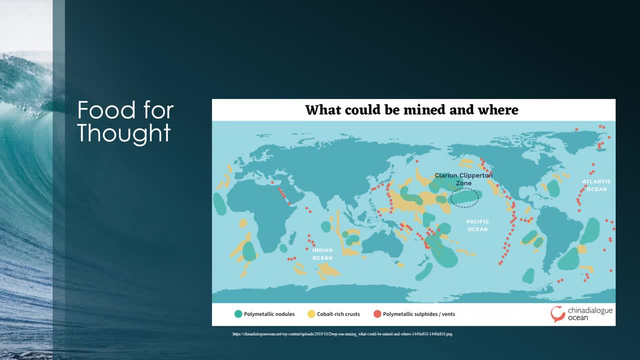 an area which demands more exploration and remains something to keep an eye on.